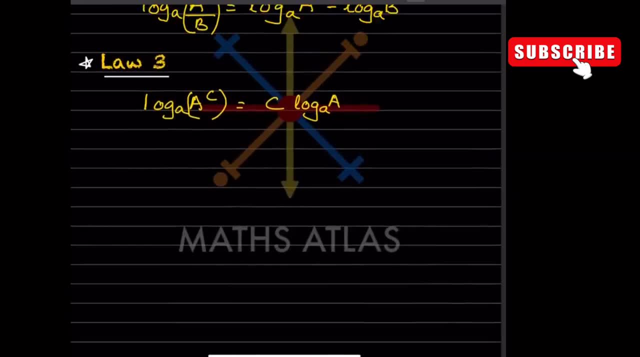 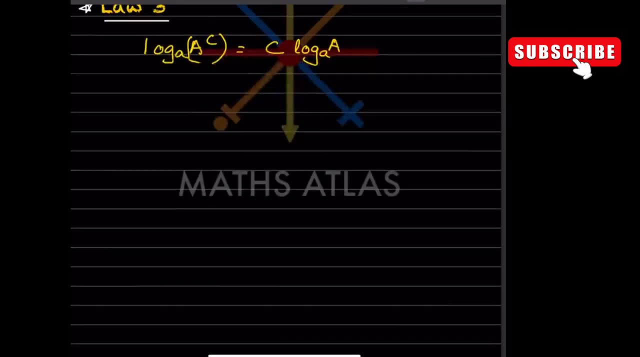 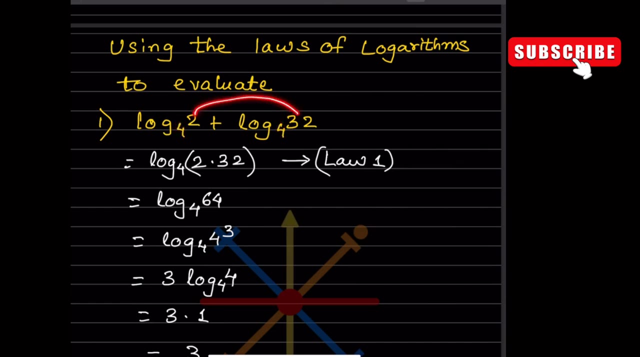 now what we can do here. this is actually addition, so you can see the law of first law. this multiplication becomes here. so this we can go in the reverse order. so what we can do here. because the base is the same for this one, so we multiply this into this one. so 2 dot means that is a multiplication, not the. 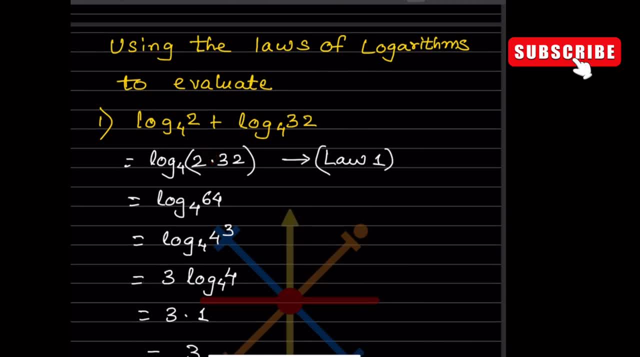 decimal. so we can also write a multiplication. so 2 into 32, to the base force it is, this is the lower one. so 32 into 2 that is going to be 64. so what we can see here, because the base is for this 64, we can also write s 4 into 4. 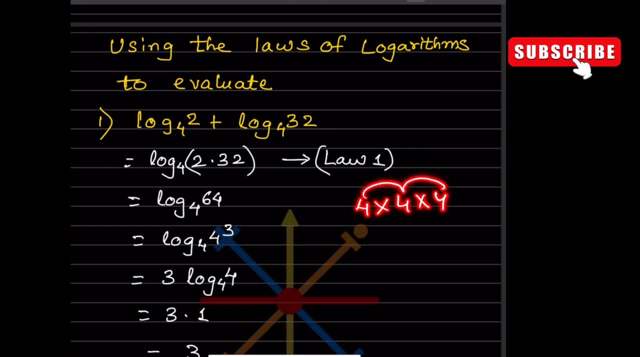 into 4, that is, 4 for the 16, 16 for the 64. so that will be 4 to the 4, s, 2, 3. so now see, here we have the law. this will go here. that is the third law 3 log of. 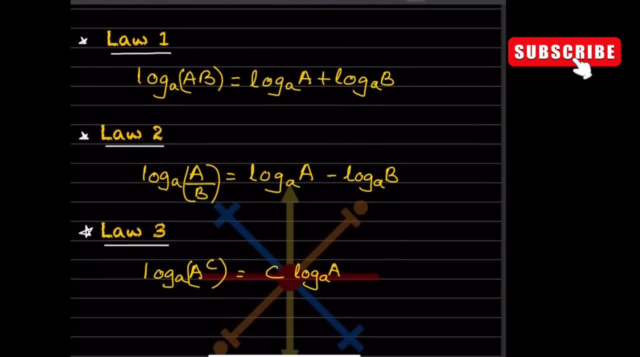 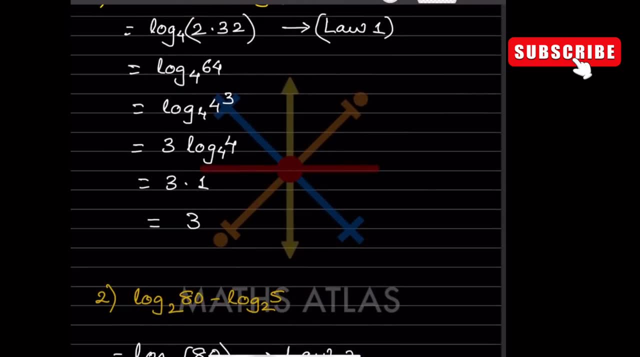 4 to the base. this is: log of 4 to the base 4. can you see the third law? this experiment goes over here, so that will be this. 3 will be as it is. so when there is the same log of 4 to the base 4, this is: 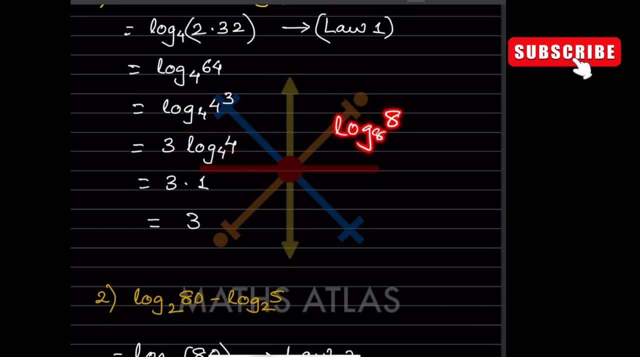 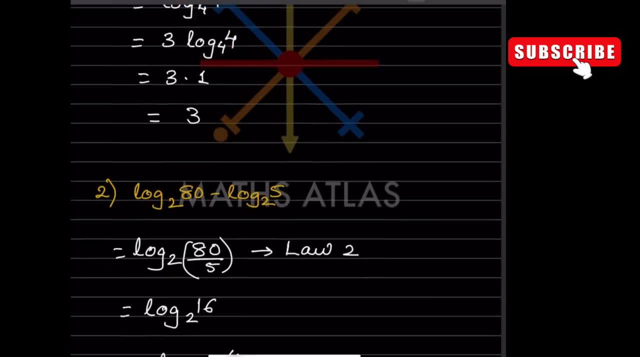 going to be 1. it can be anything. log of 8 to the base 8, so that can be 1. so if both the numbers here are the same, that is going to be 1. so 3 into 1, that is going to be 3. so now we have log of 80 minus log of 5 to the base 2, both the 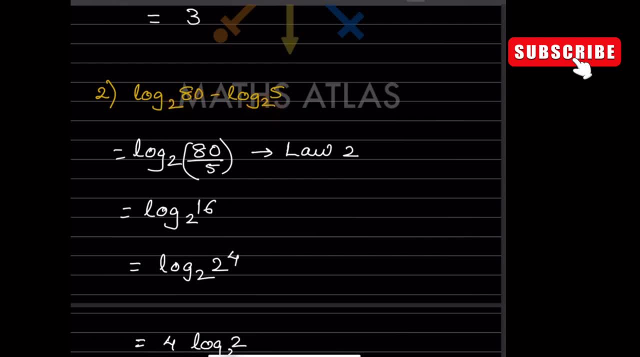 base are the same. so minus means it is going to get divided, the law 2. so this: we are going to 80 divided by 5 to the base 2. so 5 ones are 5, 16s are so here log of 16 to the base 2. so what we can write. 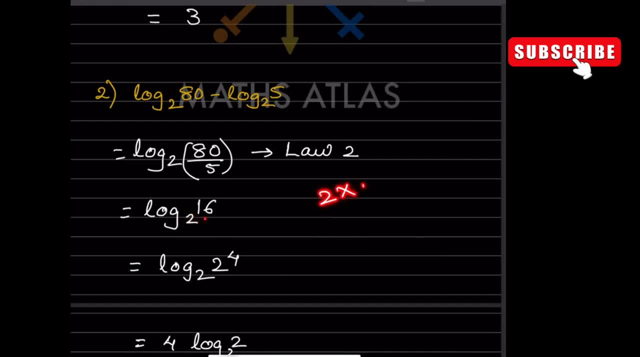 here because this is 2. we can also write this as 2 into 2, into 2 into 2. by taking the factors, that is going to be 16, 2 to the 4, 4 to the 8, 8 to the 16, so we can. 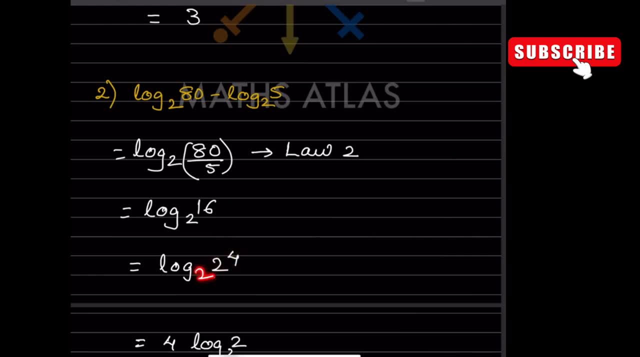 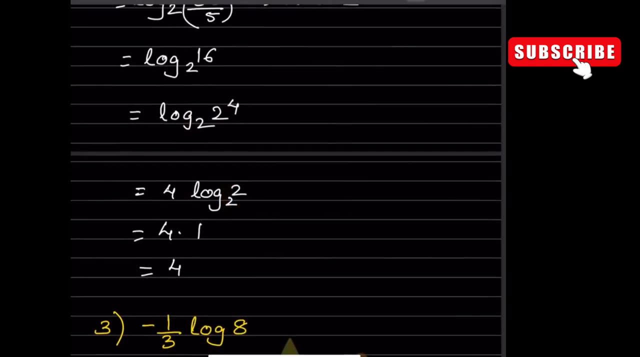 write here: 2 to the 2, raise to 4, so here to the base 2, so this 4 will go here, the third law, so this remains. so now again here, as I said, if both the numbers are same base and the year, so what we can write here. this for this whole part. we. 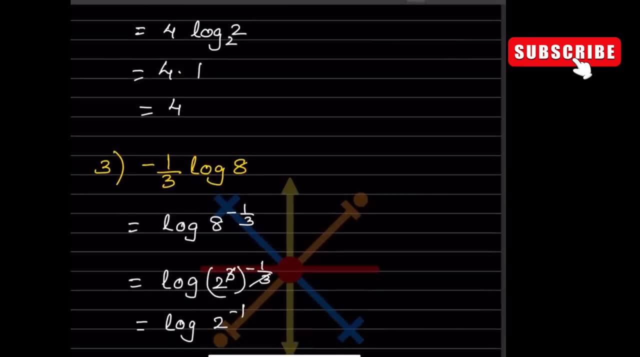 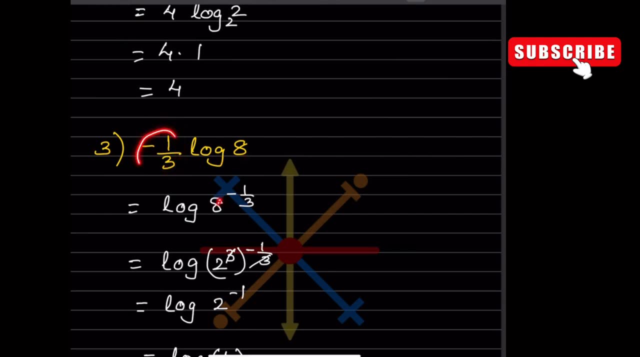 can write 1. so 4 x 1, that is going to be 4. so now what we can see here, minus 1 by 3, log of 8. so we can write a log of 8 and this, minus 1 by 3, we can write in: 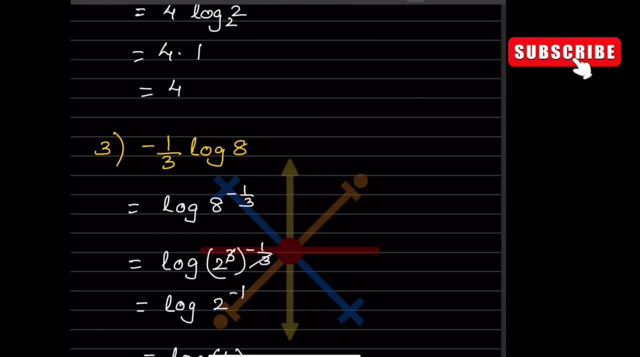 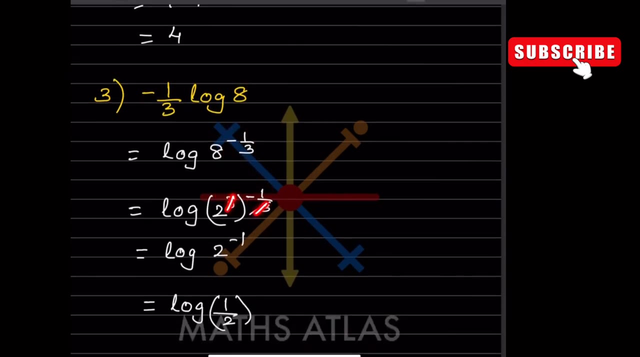 the exponent. so here again what we can do: 8. we can write 2 into 2. into 2, that will be 2 cube. so this is going to be for this one. we can write here and this: the exponent is the same. so now what we can do here. this: 3 and 3 we can cancel out. so 2 to the this. 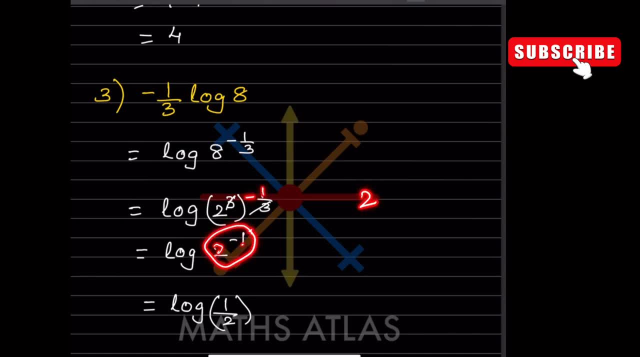 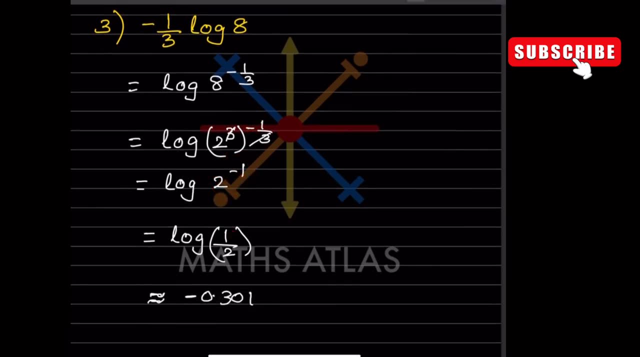 rest to 1 minus 1. so this is the. we can write this. whenever there is a inverse here, we can make it to 1 by 2. so this is 1 by 2 and when we take- you can check this with your calcine- you get the answer. 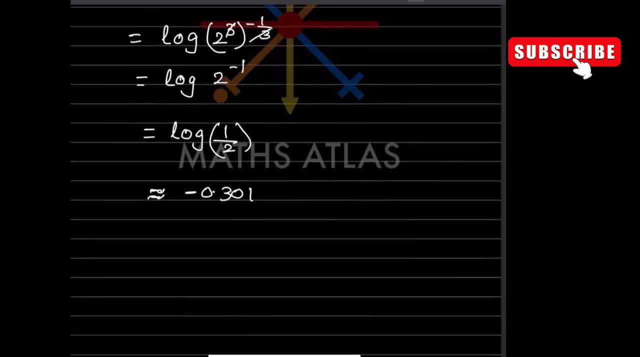 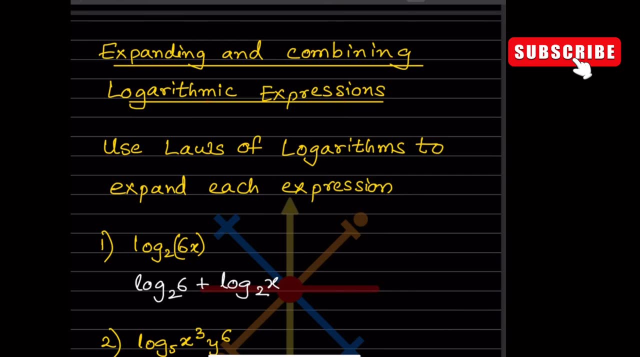 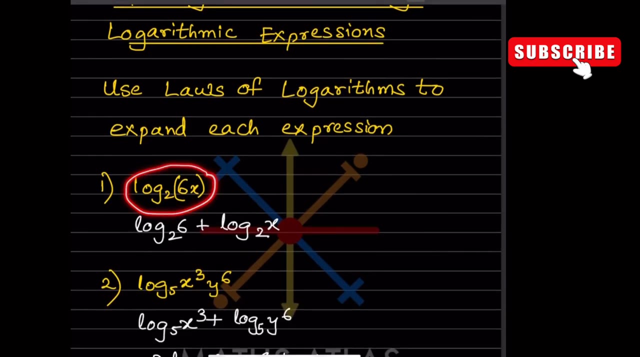 that is approximately minus 0.301. now we will see the expanding and combining the logarithmic expressions, using laws of logarithms to expand each expression. so now we can see here we can write this one: this is multiplication, so we can separate it whenever there is multiplication. 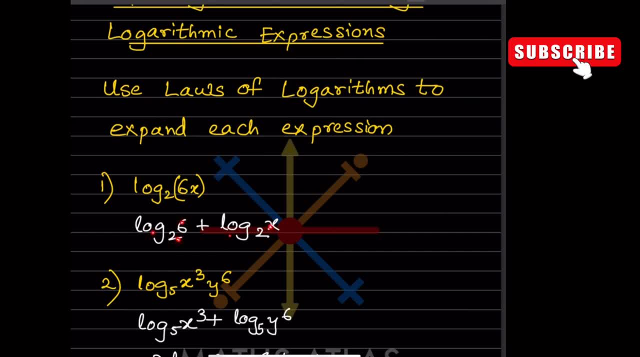 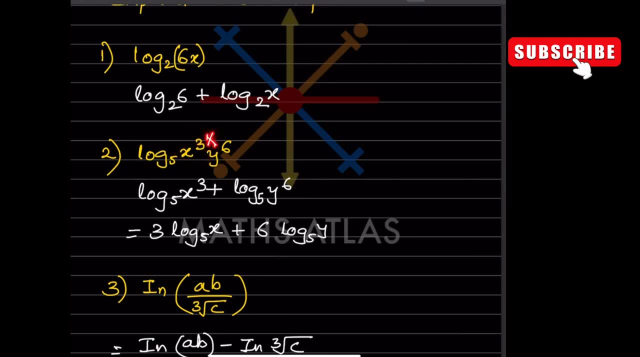 let's get added log of 6 to the base 2 plus log of x to the base 2. so this is the answer. again, this is the same. this is multiplication. so you are going to separate it, you are going to add it. so now what? 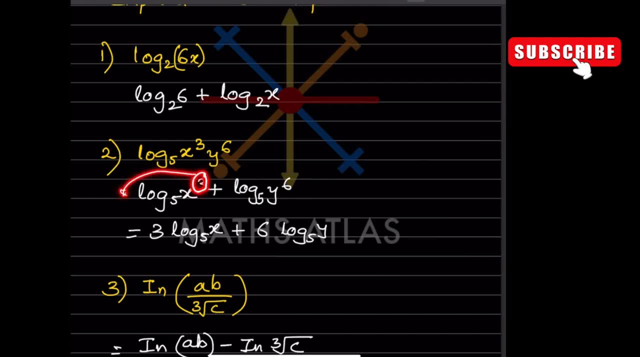 you can do further. now can you see the exponent is 3, so you can take over here. that is 3 and this will be log of x to the base 5. again here 6, you will take here. log of y to the base 5, you will. 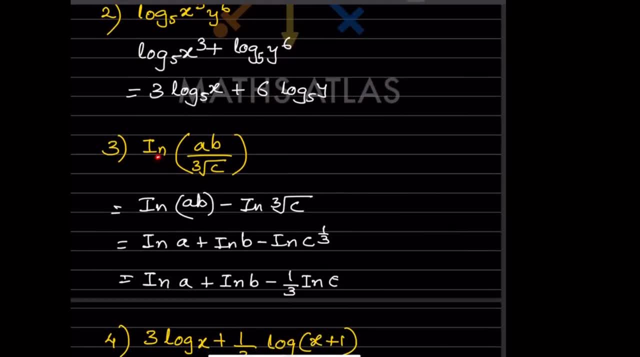 write here. so this is the answer. now this is in. this is actually the natural logarithm. i n so we can write here: this is division means you are going to subtract it. i n this will be a, b minus. i n this will be root of cube. 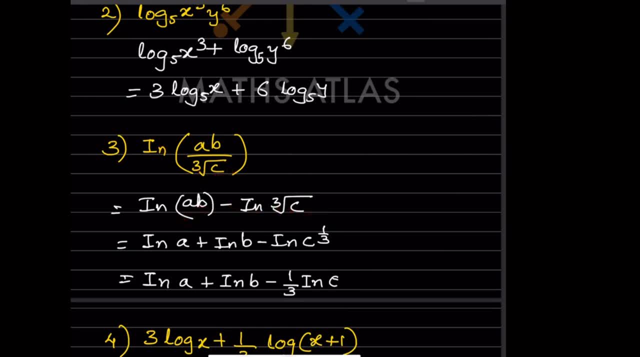 root of c. so now we can write this one, as this is actually multiplication, so we can write this. we can add this minus this one. so now again, this remains the same, so we can again further what we can do here. 1 by 3 in this is c, so this is the multiplication. so 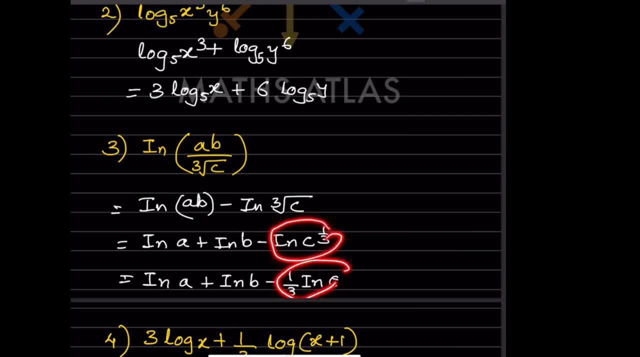 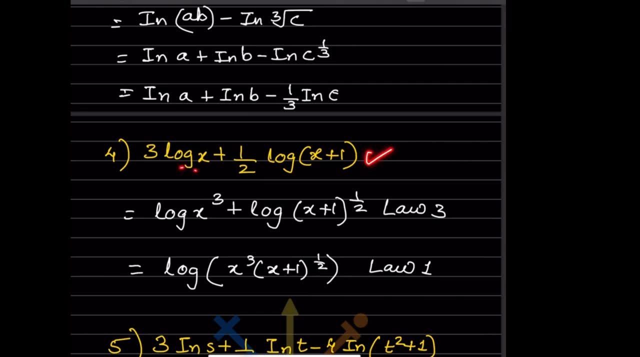 we can also write this as log of x. that is the second part. so this is the third log for this part. so this is the answer. so here we can write here: this is for 3, log of x plus half, log of x plus 1, so we can also write this as log of x and this will be cube for 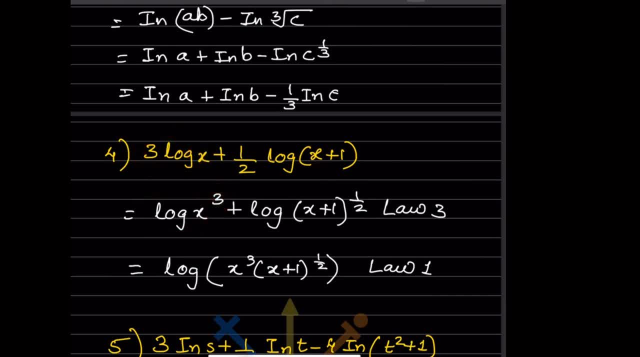 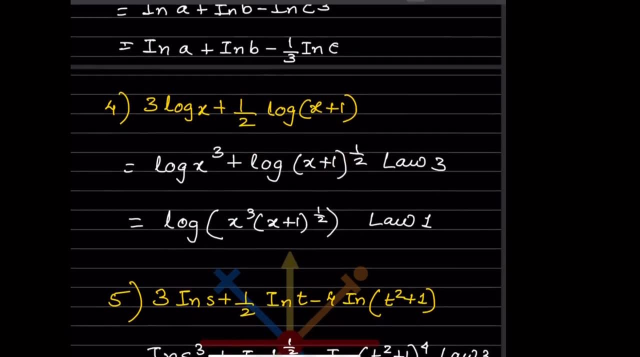 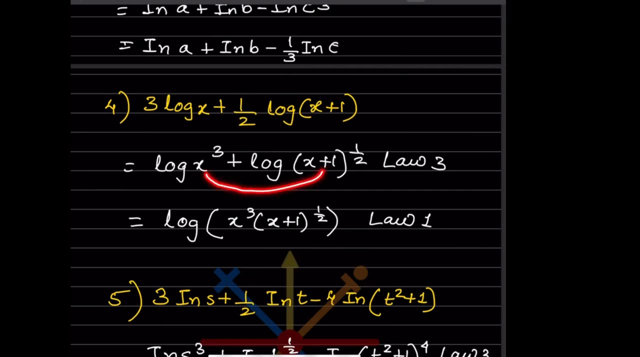 this part. so again, for this part we can write here: this whole thing will be as it is and this one by 2 will be in the exponent, which is the law 3. so now, what we can do here. we can do here: this is plus, so we can also multiply by the log 1, so this into this part. so x cube. 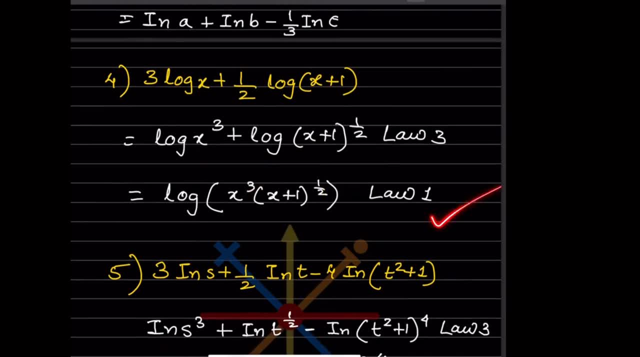 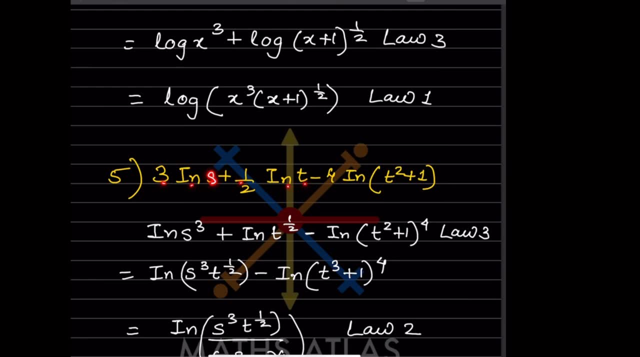 into x plus 1, raise to half. that is log 1. so this is the answer now for this one. 3 in this is s plus half in t minus 4 in t square plus 1. so for this one we can write here: and this 3 will go in the exponent. here again we can write this part, this half will go in. 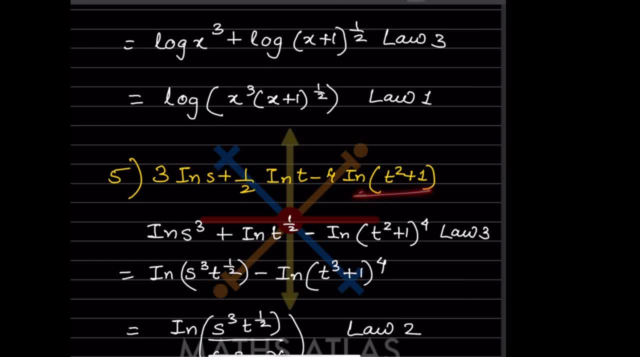 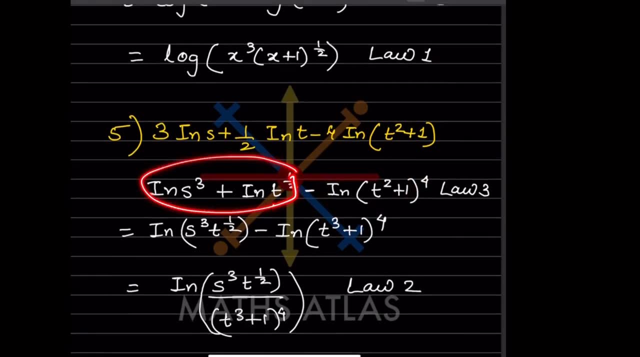 the exponent 1 again. we can write this whole thing over here, and 4 will go in the exponent, that is the log 3. so now what we can do here here. this is plus, so we can multiply it, so this into this one. n is here outside again for this one. this will keep this whole part. 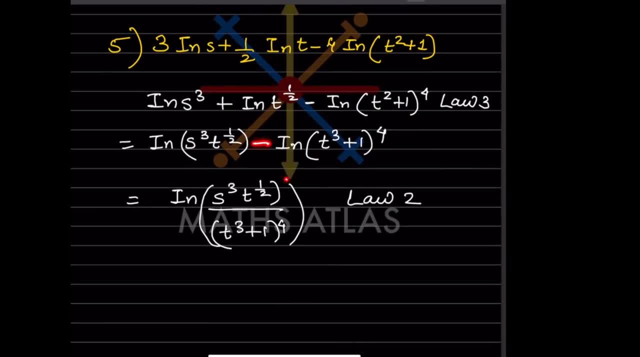 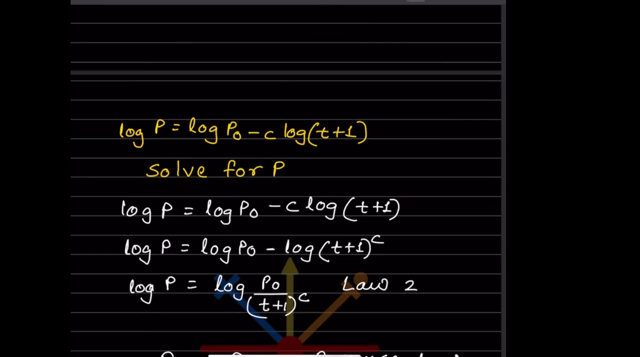 the same. so now here this is subtraction means it is going to get divided. So this fourth are in here. so this divided by this part. so this is so. this is the log 2. so this is the answer. now you, log of p is log of p of 0 minus c, log of t plus 1 and. 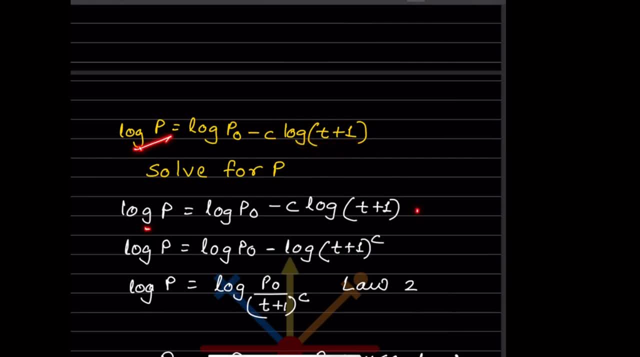 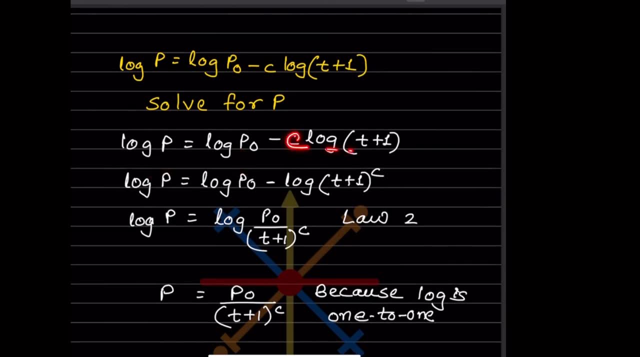 you have to solve for p, so this will keep. this will be same. we have repeated location over here, same, So for this one c log of this means we can put this: Okay, see, in the exponent. so this will write same and this will go in the exponent here. so now what? 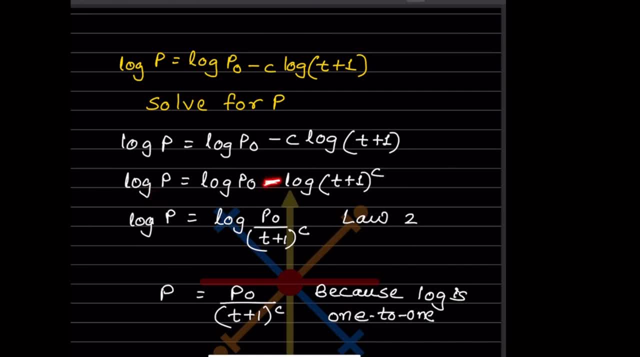 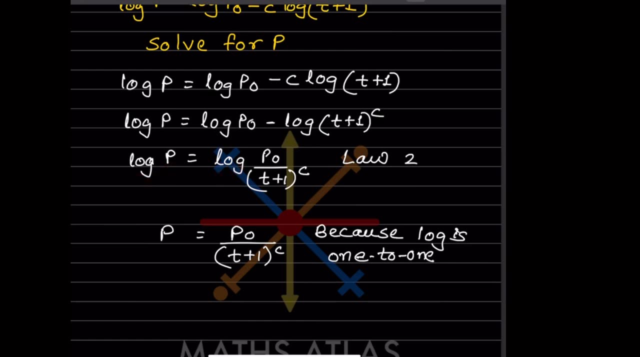 will you do? log of p is equal to now. can you see? here is subtraction. so both side log means you are going to write it once and this is going to get this part. both of them are going to get divided according to log 2. so now we just want p. both the sides we have log. so what log is actually? 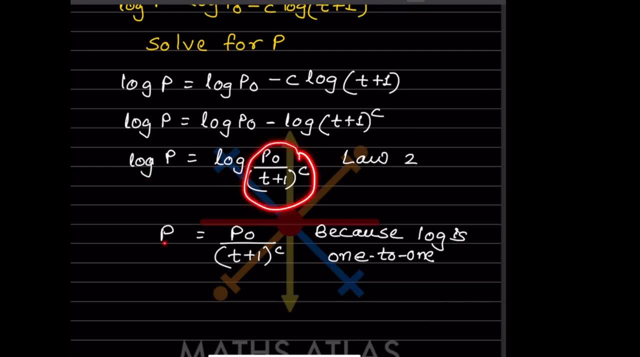 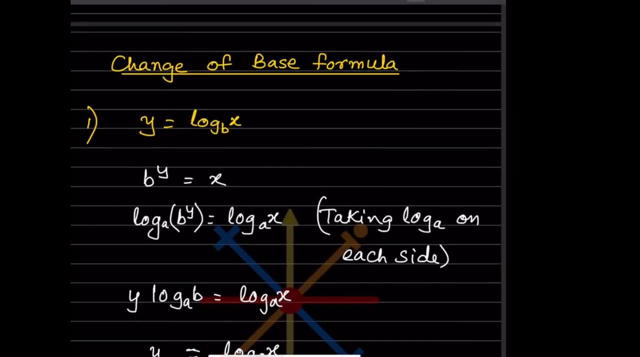 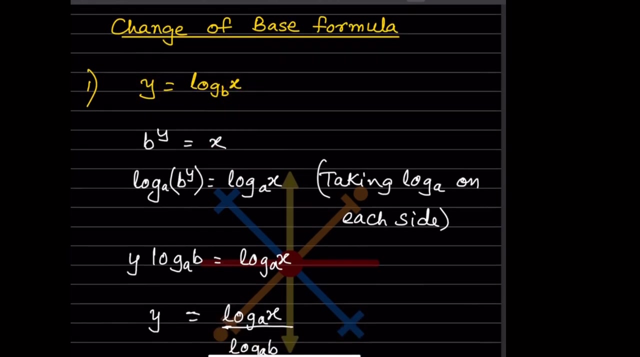 one by one. so what we can do, p is this one. so this is the answer. now we have to see how to change the base formula. so y is log of x to the base b, so we can also write this one, this base. so this one, when we b raised to y, is equal to just x. so now here, what will you do when we take: 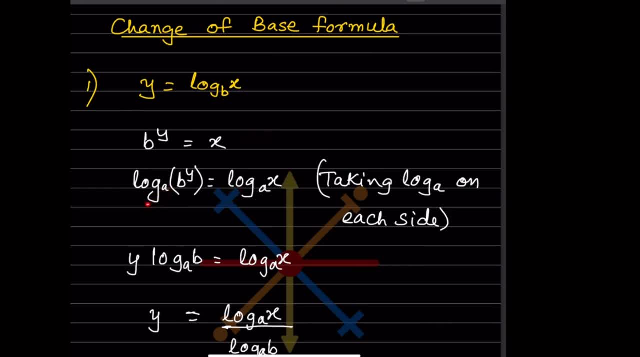 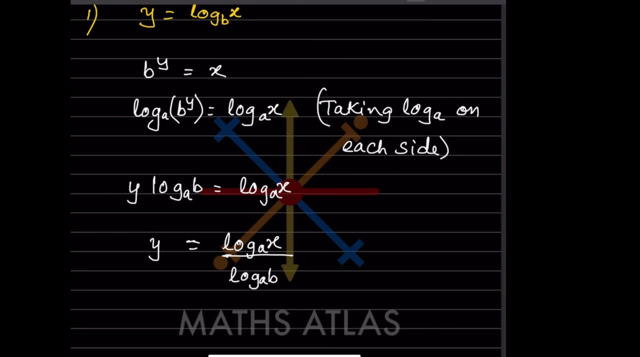 log on both sides for this expression. so what will you write here? so log of b to the base b, b raise to y to the base a is equal to log of x to the base a. so taking log of a on each side. so what will we get here? this will go here. so that will be y, this whole thing. 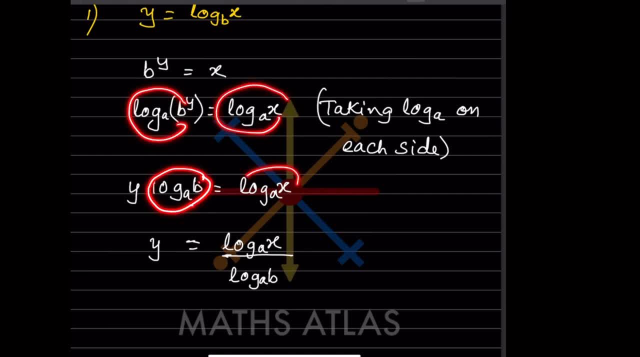 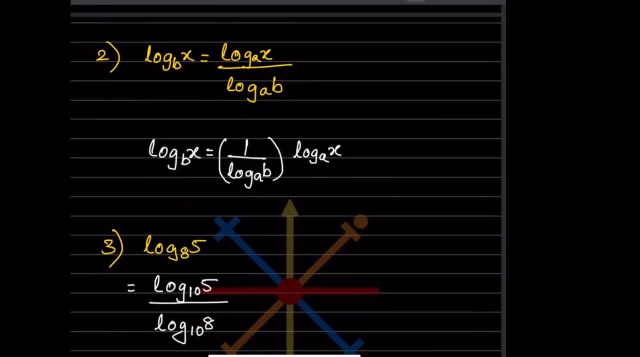 will be here: log of b to the base a and this is the same. so we will find the value of y, so y will be: this is the same. but this is actually multiplication, so this is going to get divided, so this will go here. so this is the answer. again, here we will solve for this part. 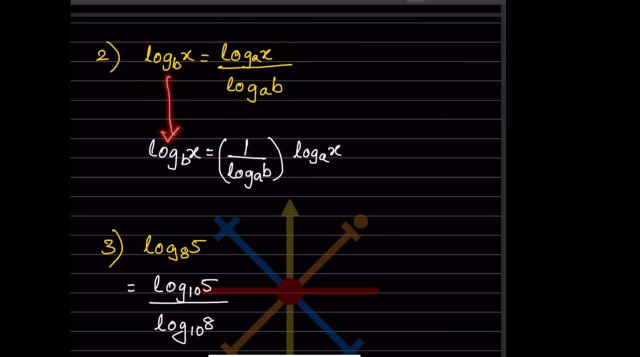 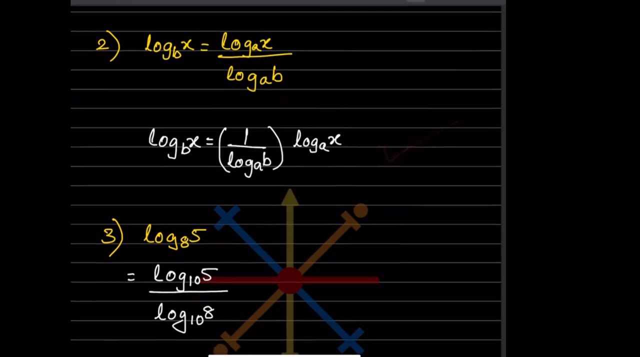 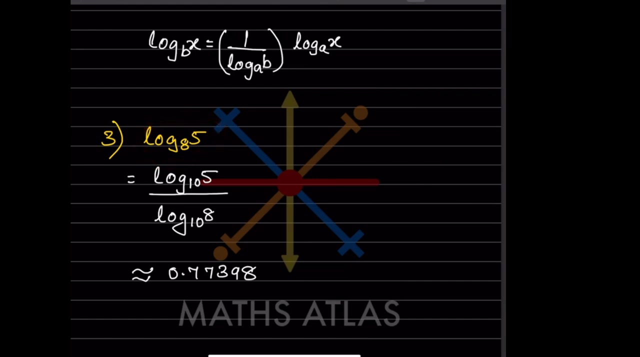 so this will remain as it is and here we can separate this one. so you can also write a 1 by log of b to the base a and this is log of x to the base a. this numerator as it is, this is the answer. now, look at here for this one we can write: here we can take the base as 10, so what we can write. 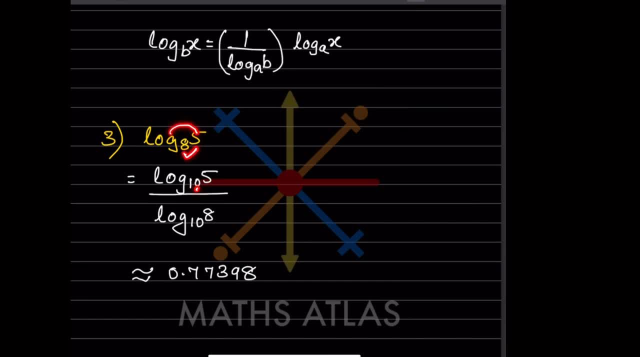 here log of 5 to the base 10 and this one log of 8 to the base 10. so when you, you can look in your calc, because this we cannot do it directly. so you get the. when you divide this one, you get this answer. this is the approximate answer. 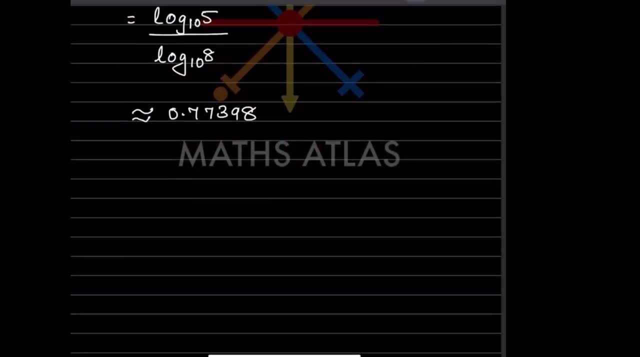 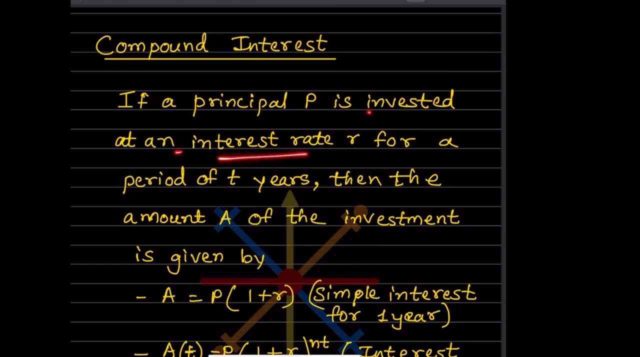 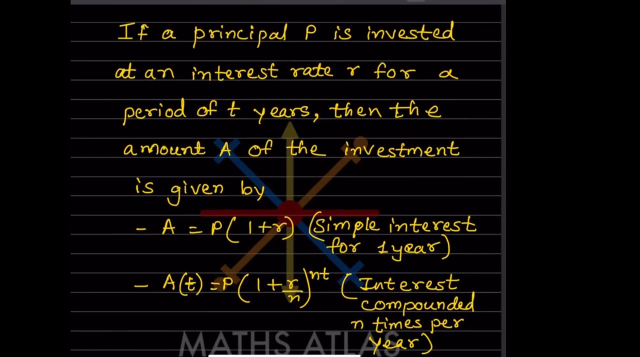 when you write like this means that is the approximate answer. now we will see for the compound interest here. if a principal p is invested at an interest rate r for a period of t years, then the amount a of the investment is given by. so whenever there is for one year means we write this formula: a is equal to p into 1 plus r. whenever the interest 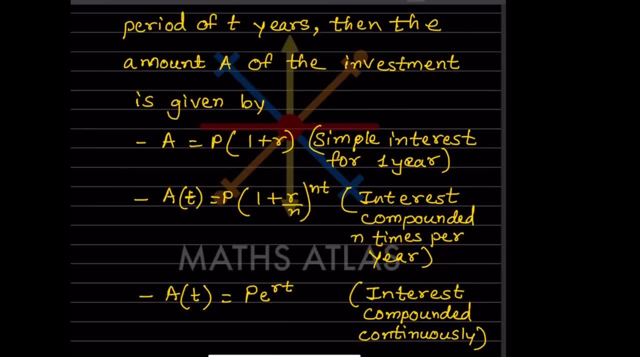 compounded, that is n number of times per year, that will be a into p, that is, p into 1 plus r is to r divided by 2. so this is the amount a of the investment is given by. so whenever there is for, n is to and nt, and when the interest compounded continuously. so we have, we have this formula. so 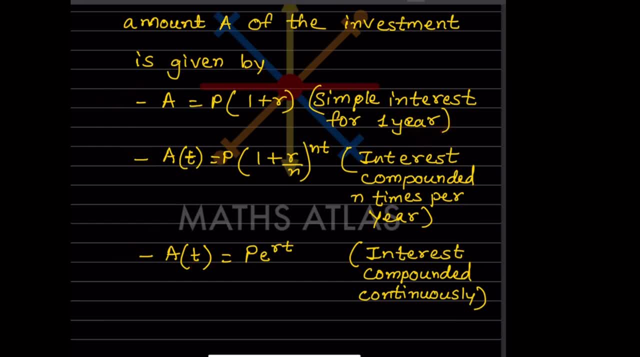 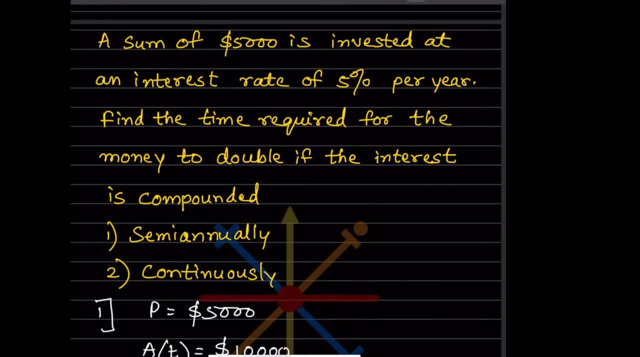 you have to remember all these three formulas for one year, for n times per year, and that is continuously so. now let us see the problem here. a sum of dollar 5000 is invested at an interest rate of five percent per year. per year it is given here. find the time required for the money to double. 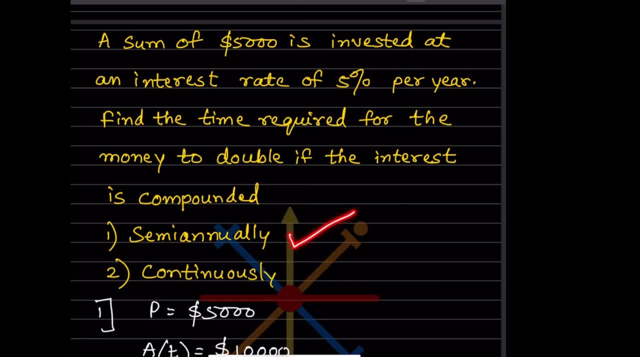 if the interest is compounded, and the interest is compounded, and the interest is compounded, and the interest is compounded. so we have to see, if it is semi-annually means here half, and this is going to be continuously. so now first let us see, for semi-annually so, what is given whenever the sum of dollar 500 means the 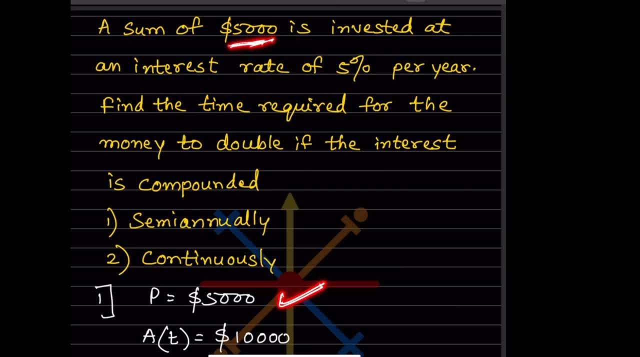 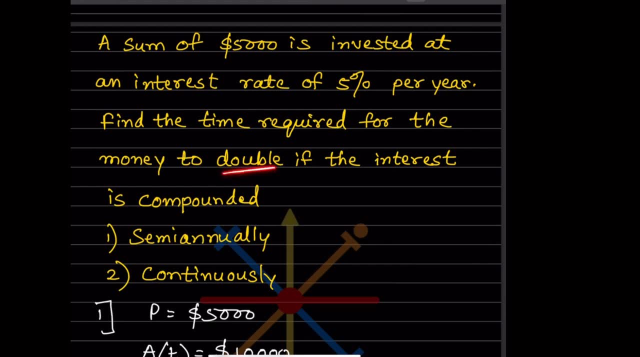 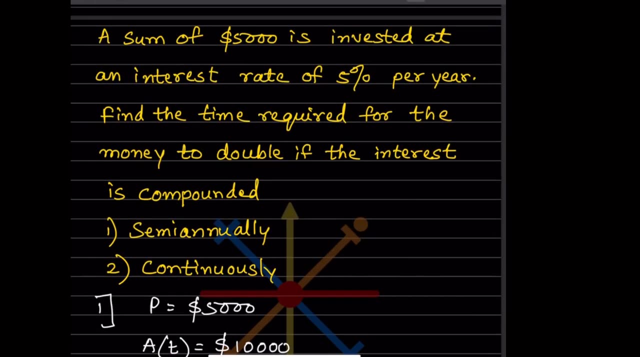 principal is given is so sorry. it is 5000 means it principal is given as 5000. and then it find the time required for the money to double. double means here. this is the time required for the money to double. amount will be 10,000. and what is are given? the rate is given as 5%. so whenever we have 5% per year, 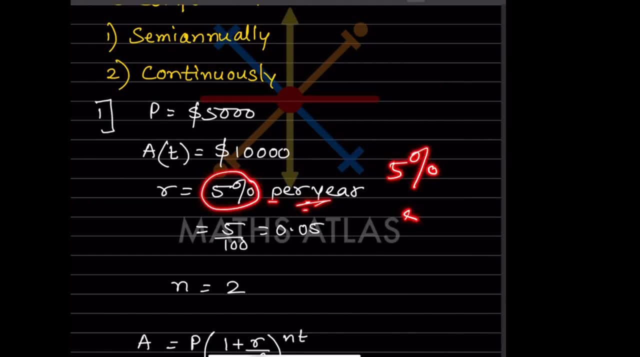 so 5% means we, whenever you have this sign, that means we write 5 and this sign means this is going to get divided. so 5 divided by 100, and that is going to be, you know, whenever there are two zeros means you will write this 5 and then you will go backwards by two number and then put a decimal. so 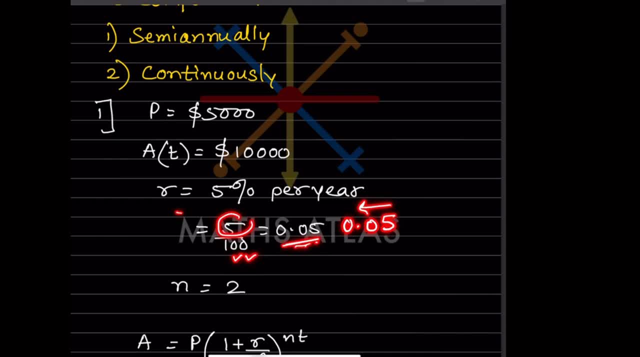 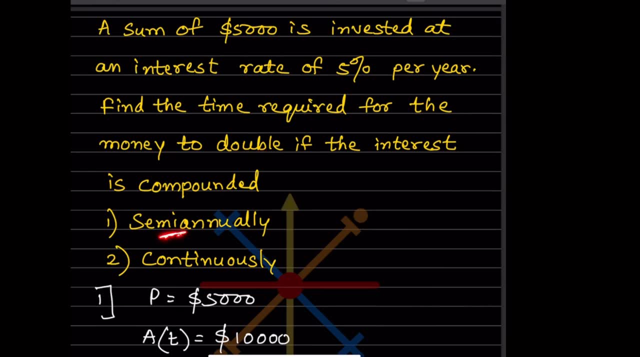 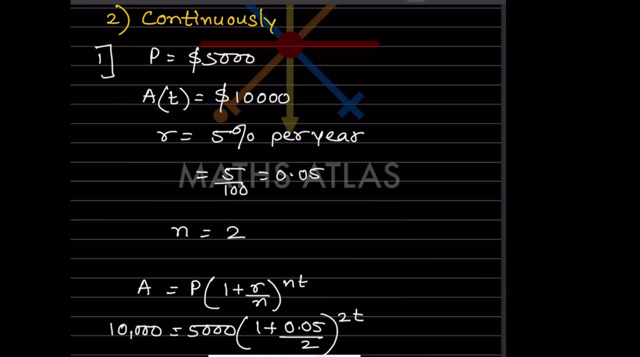 that will be 0.05. so r is 0.05, and here, if it is going to double, means here, here it is. now it's given here semi-annually, whenever the semi-annually means two times, n times. so this is going to be n is going to be two. so now we have. 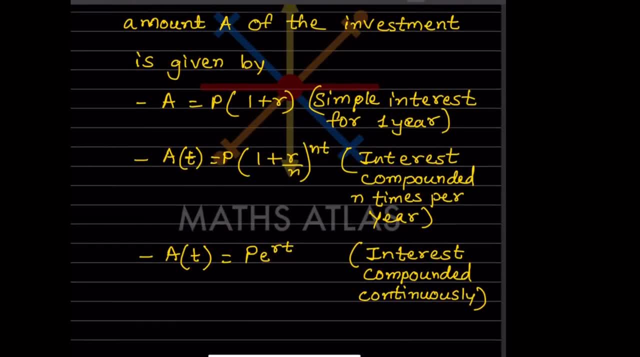 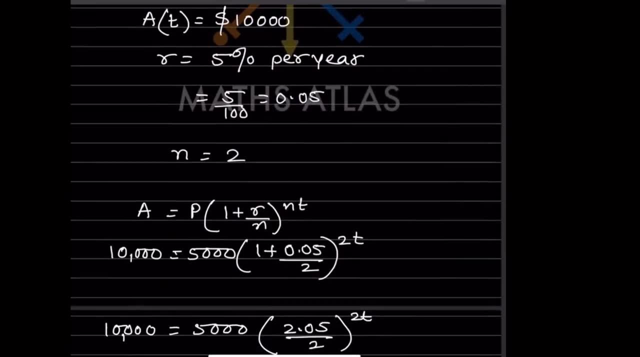 a formula for this one, so we are going to use this one. because interest compounded and n times per year, so we are going to use the second formula. so here, a is equal to p into 1 plus r, by n, rest to n t. so now we have the amount. 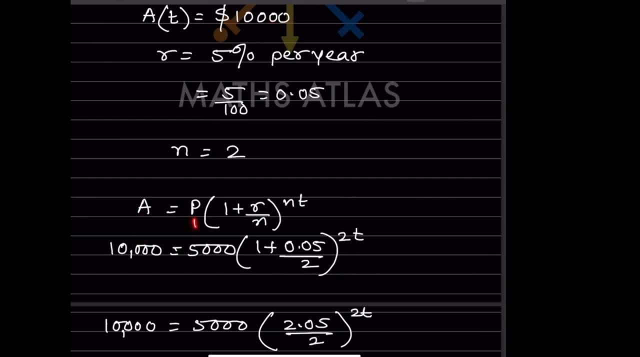 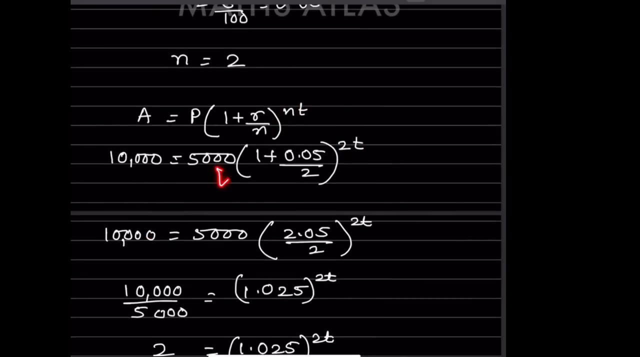 that is 10,000. so we are going to put below this 10,000 principal 5,000. so 1 plus r. what is r is given here 0.05, and n is 2, and here n is 2 and we have to find out t. so here let us write the same. 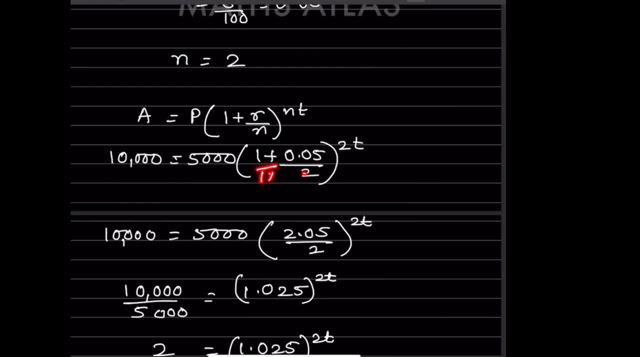 so now, here, what we can do here is 1, so you will take 2, so you take the LCM of that. so this is going to be t plus 0.05, that is going to be 2.05 divided by 2. so now, how is that going to be this? 2t will be same. so now, when you 10,000 is here and this is: 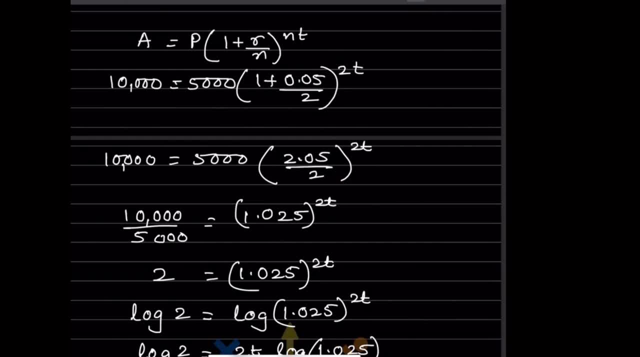 multiplication, so this can be divided. so we will take this on the other side. so here, when you divide this one, 2.05 divided by 2, you get 1.025. this 2t as it is, so now this will be this- gets cancelled. 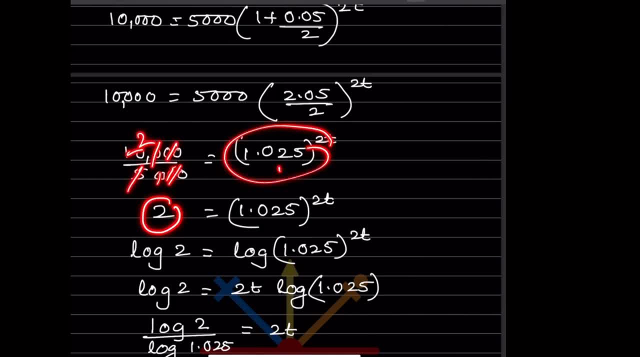 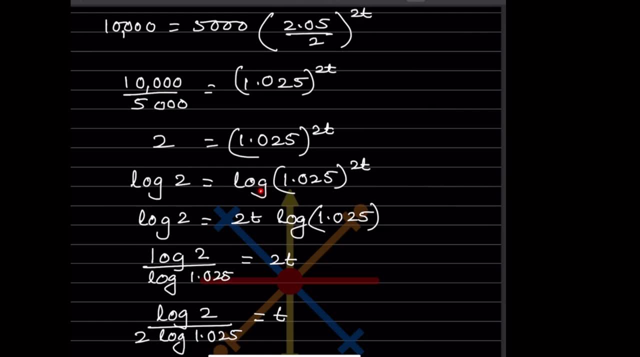 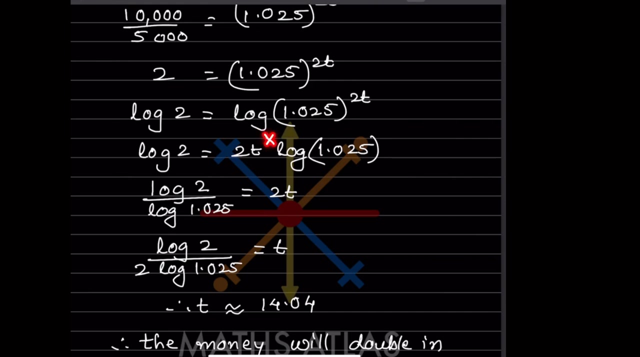 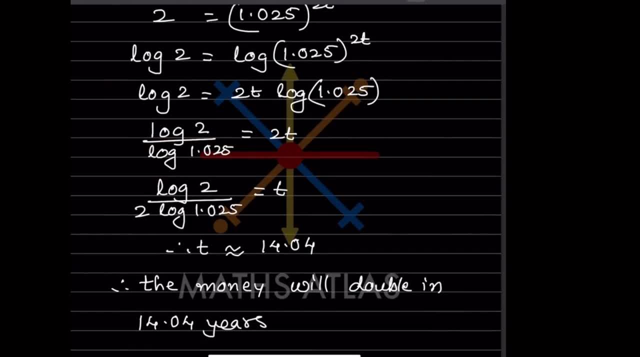 to get divided and this 2t will be here, but we don't want 2t, but we just want t. so this 2 we will take on the other side. so this is going to get divided, whereas this is going to be the same. so now we just calculate with the others. you can use a calc over here and 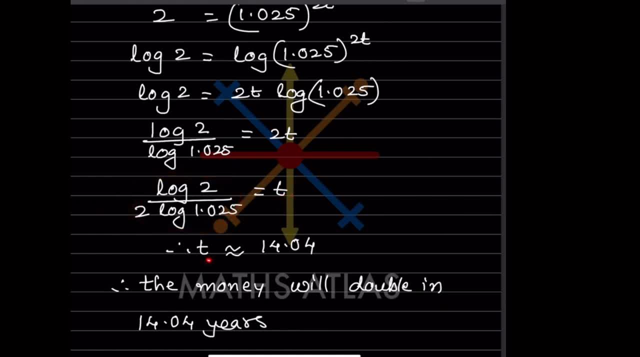 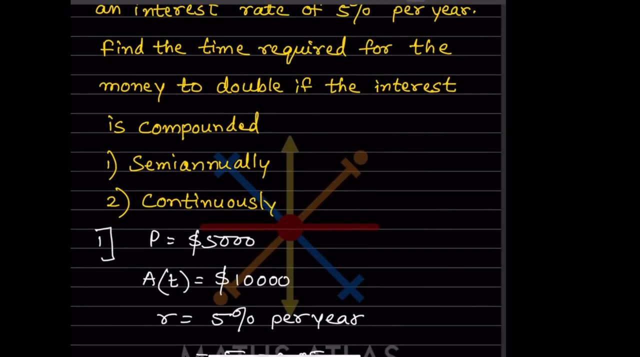 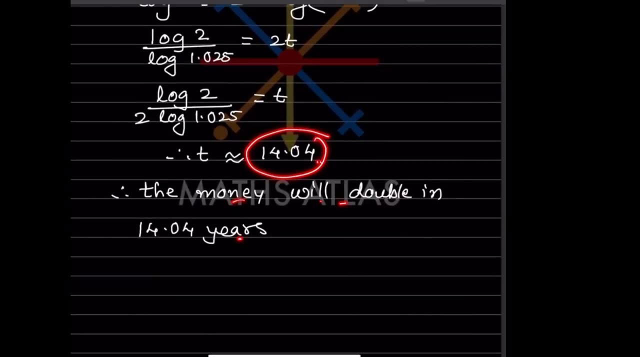 you can just put the values, this value, so what you get is t, is approximately, that is 14.04. so what did they ask here? find the time required for the money to double. so here, therefore, then money will double in. this will be 14.04. that is years. 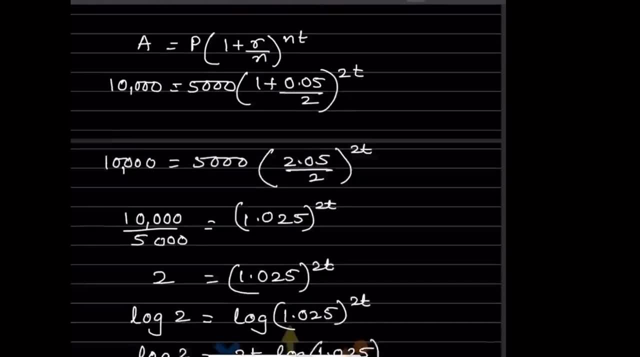 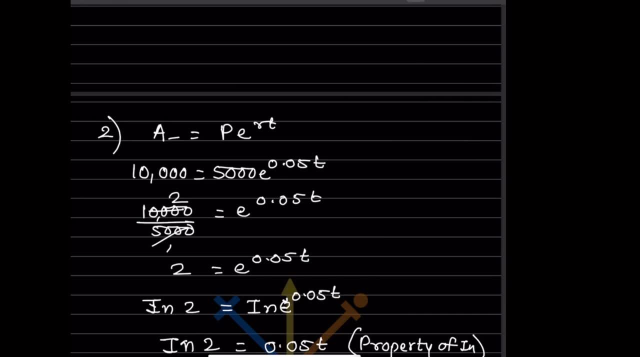 and now we will use the second one, that is, for the continuous list. so we have the formula for the continuous list that is: A is equal to. this is the formula A1, P x, A1 is equal to 14.04, that is, 14.40avors. here, 14.40 is 14.40. this is the repeat, the 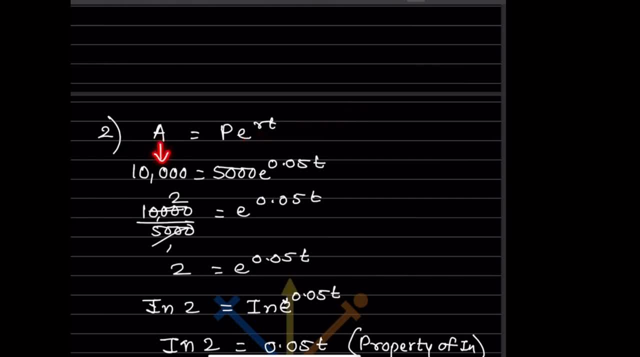 e into r is to t, so now amount is 10 000, p means the principle is 5000. e is true. now, rate of interest: we are already seen in the previous one, that is 0.05, and this t is going to be the same. so now, 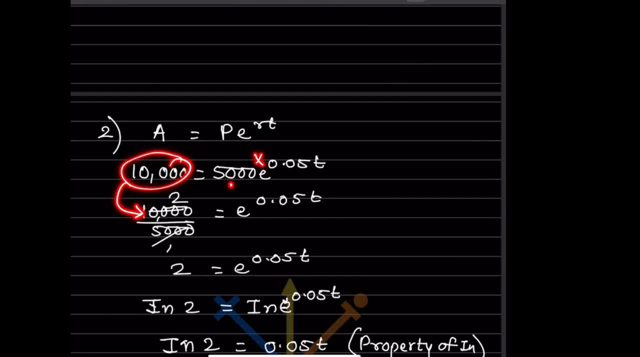 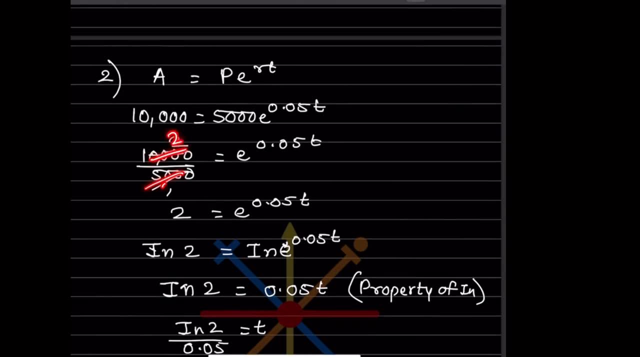 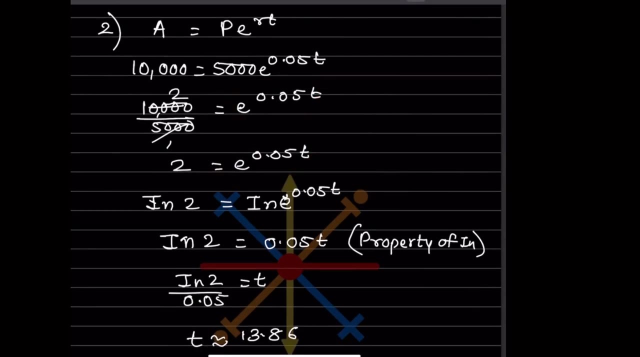 this is all multiplication, so this will be here and this is going to go in the denominator. the rest will be the same. so this: when this will be 2000, this will be 2. this is going to be the same. so now what we will do. we put in on both side. that is the property of in. so that is i. 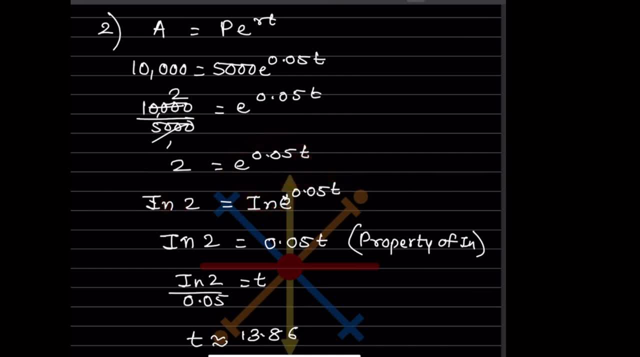 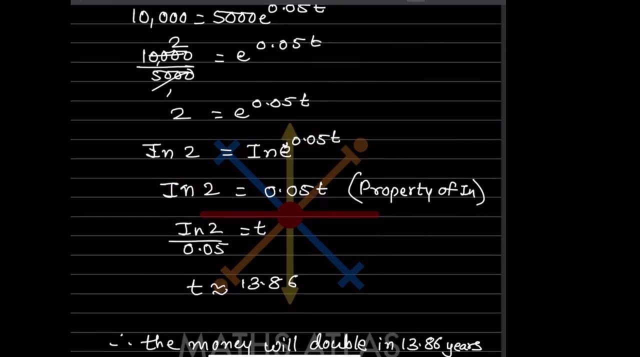 iron over here and this for this as well. so now what we can do here: when you take, this will go this side, so that will be 0.05 t. so here now what will be here: this i and this one. this will be on the left hand side, so this is going to get divided. that is t. so again, you can see this one. 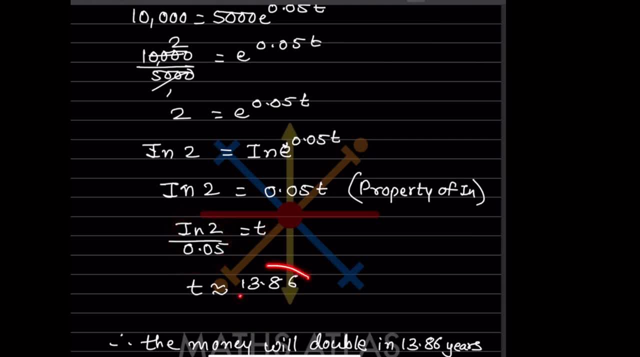 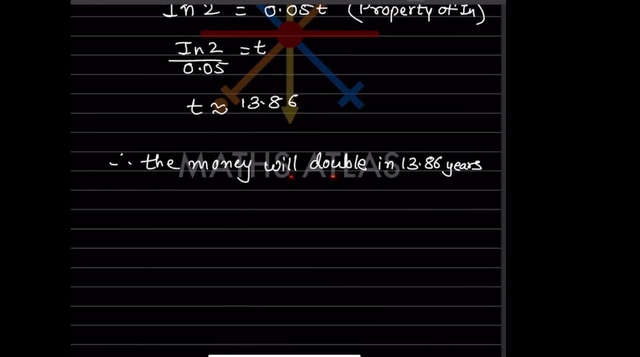 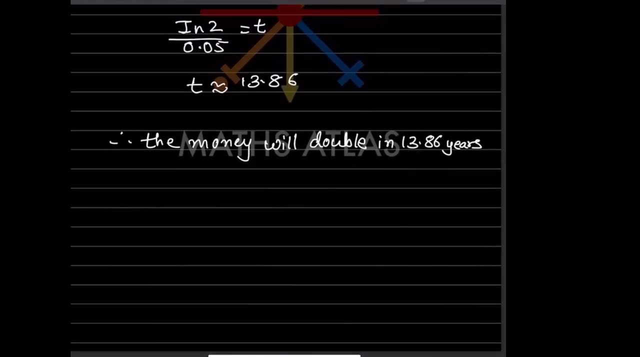 the value using your can see. so the t value is 13.86. so therefore the money will double in 13.86 years. so by this one we have completed today's work. please do like and subscribe to my channel so you get the notification of the other parts. thank you. 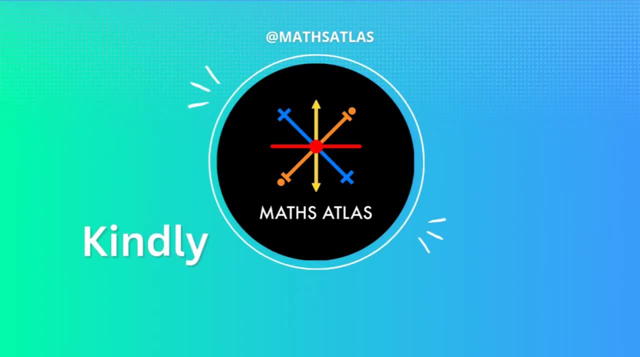 and i will see you in the next video. 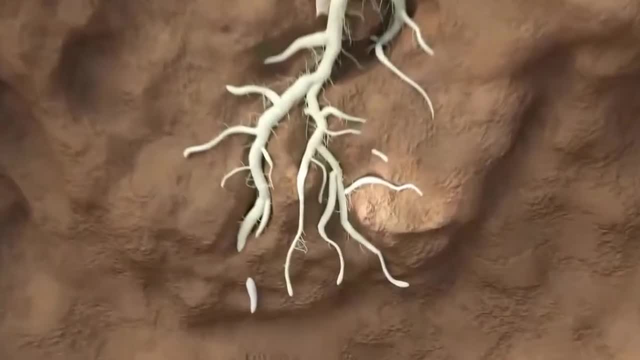 Nematodes are responsible for heavy yield and crop losses in fruits and vegetables all over the globe. Tiny eelworms, like the root knot nematode, live in the soil and the larvae, attack plant roots. Nematodes penetrate the root, start to reproduce and cause root galling. 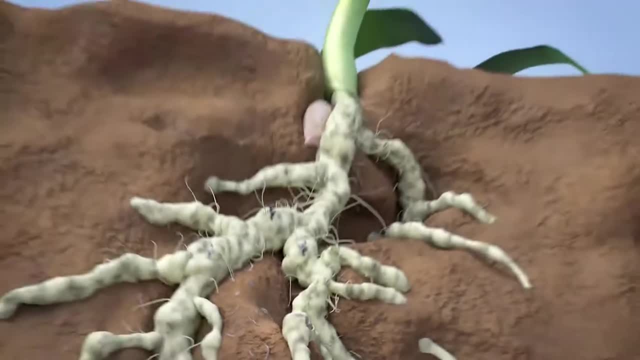 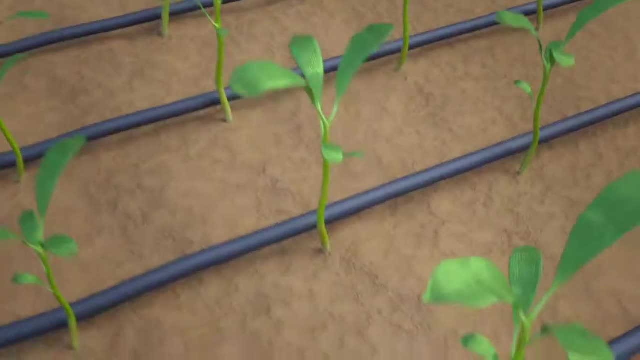 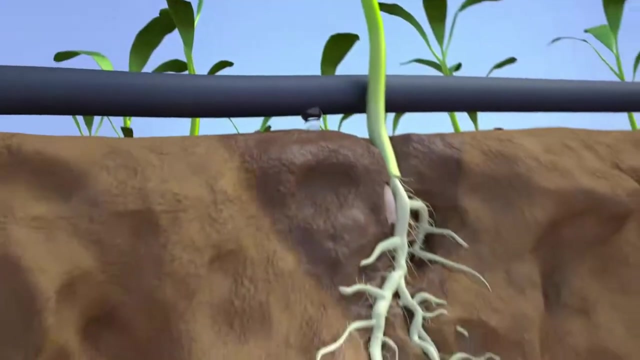 They suck water and nutrients from the root system. Infested plants suffer and show poor growth. Fluopuram from Bayer stops the attack. The active substance is applied to the soil via a drip irrigation system, allowing it to precisely target the root system.